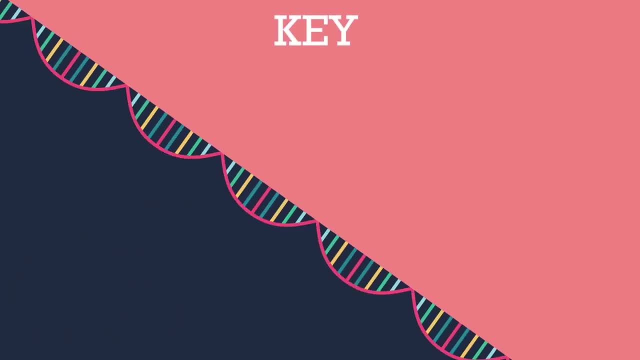 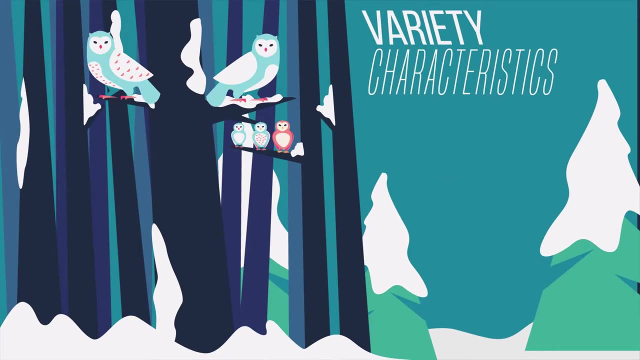 lot of genetic variation. What's the problem? The problem is that the key to having a healthy population is genetic variation. Within a population. you need a large variety of different characteristics so that a species can adapt if there is a change in the environment and avoid becoming extinct. 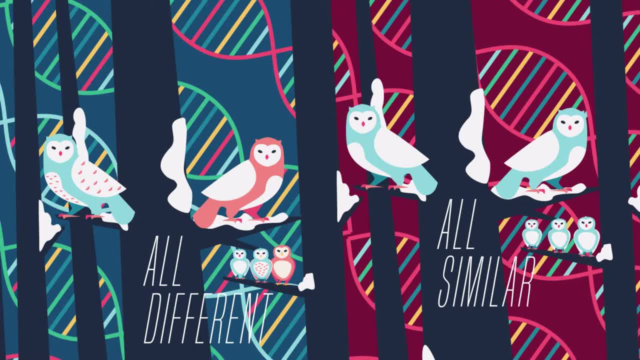 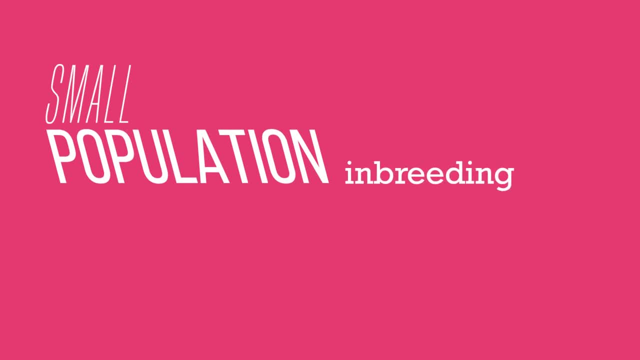 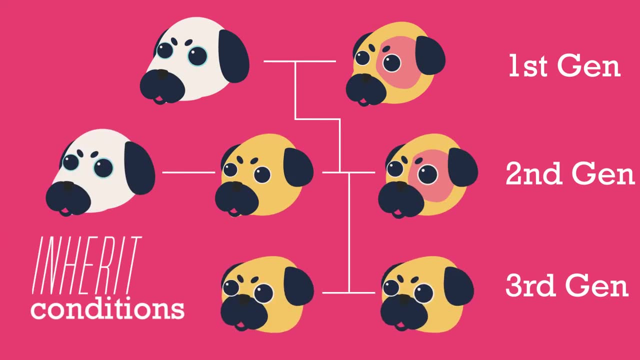 This can happen if all the members of the species have similar genes. Also, in a small population, there is a high chance of inbreeding. where closely related individuals breed, this can increase the risk of offspring having inherited conditions. so large wild populations are important for a species survival. there are many reasons why. 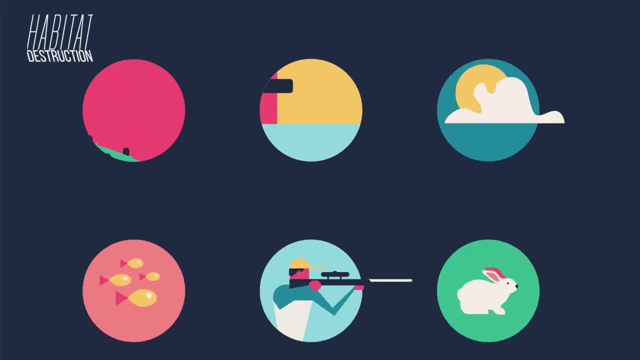 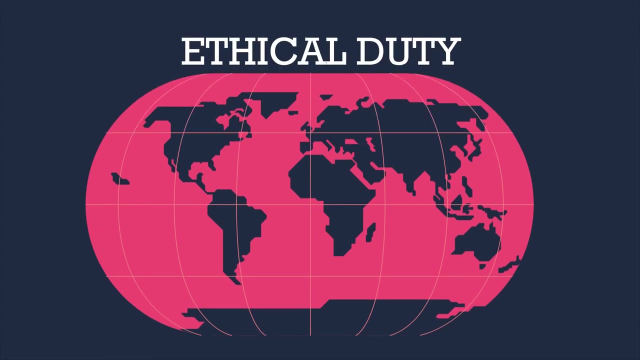 a species might become endangered. it can happen because of habitat destruction, climate change over fishing or hunting, and the introduction of invasive species to habitats which outcompete the native ones. we have an ethical duty to help preserve all the species on earth, and this is done by carrying out conservation. let's look at a few methods used. firstly, endangered animals can. 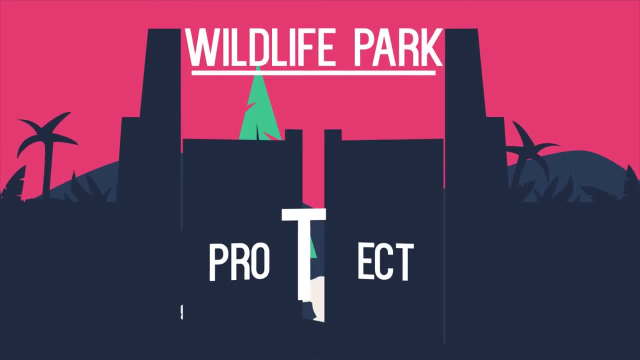 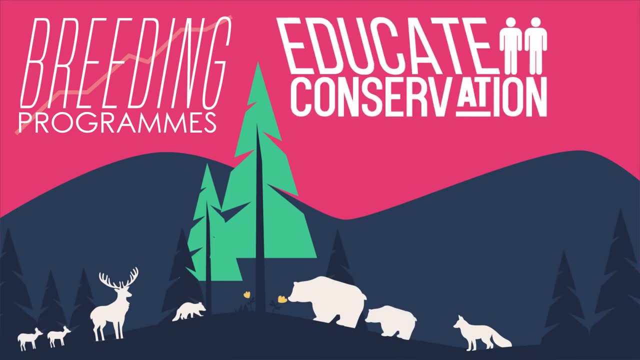 be housed in wildlife parks. this protects them and also captive breeding programs can be used to increase their numbers. they help educate people about conservation and how we can all help protect endangered species. they also help the general public to form an emotional connection to these endangered species. however, 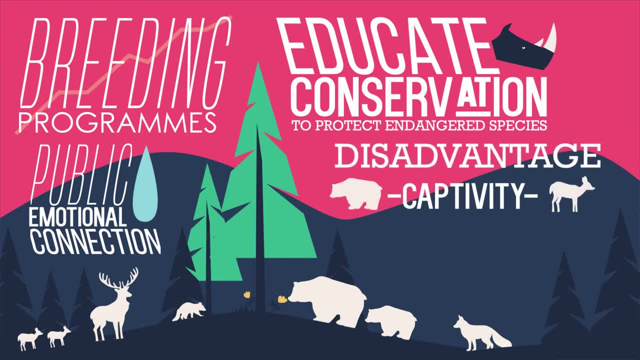 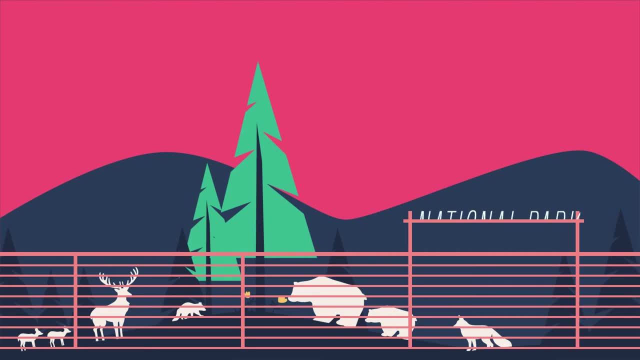 there are disadvantages to animals in captivity. the animals do not lead a normal life and there is risk of inbreeding. a way of protecting animals in their natural habitat is by creating protected areas like national parks. trees cannot be cut down, roads and houses can't be built and hunting 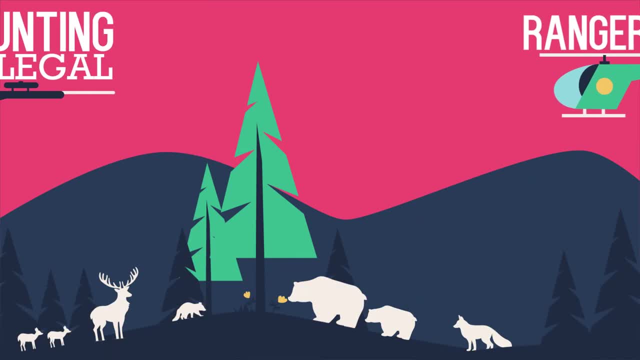 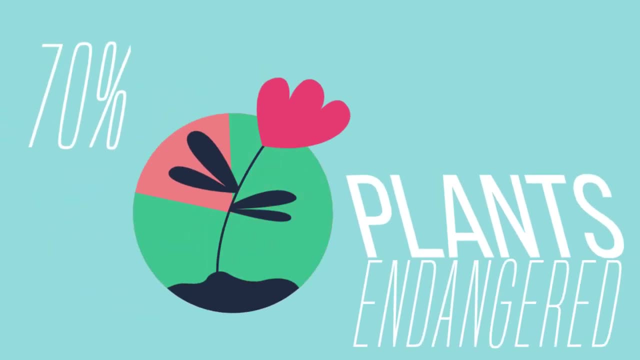 of the animals is illegal. rangers are employed to make sure this is enforced. it's not just animals: plants are also at risk. an amazing 70 percent of plant species are endangered. so it's vital that we help protect the animals. we can't just keep them in the wild. we can't just keep them in the wild. 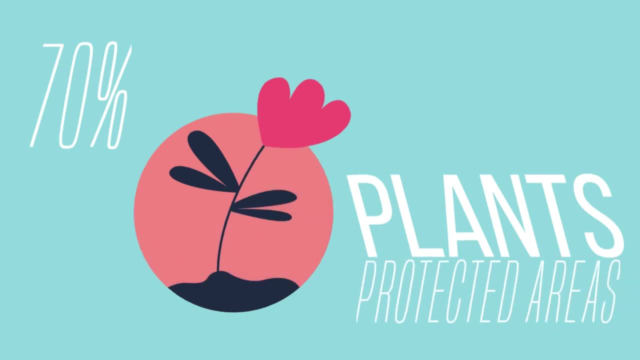 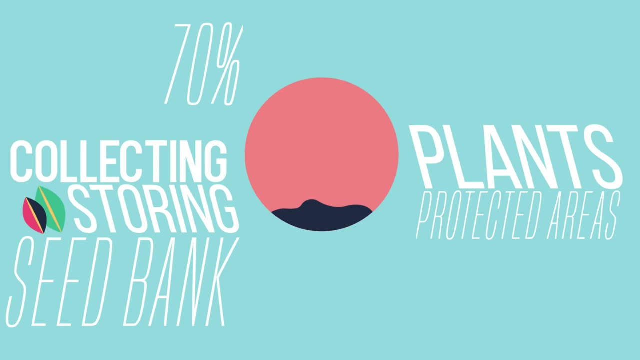 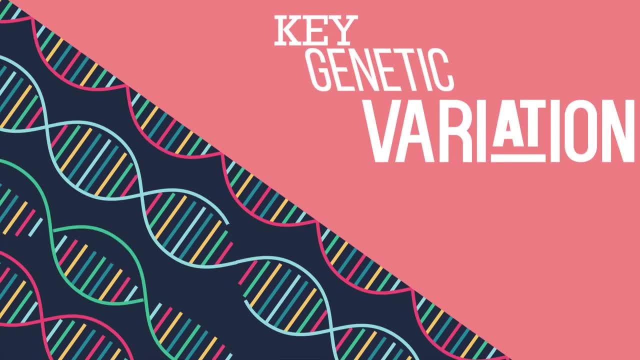 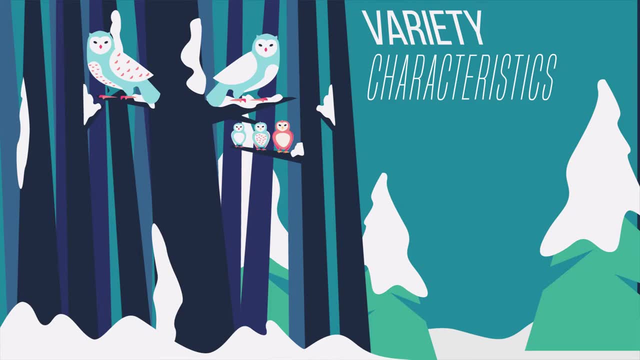 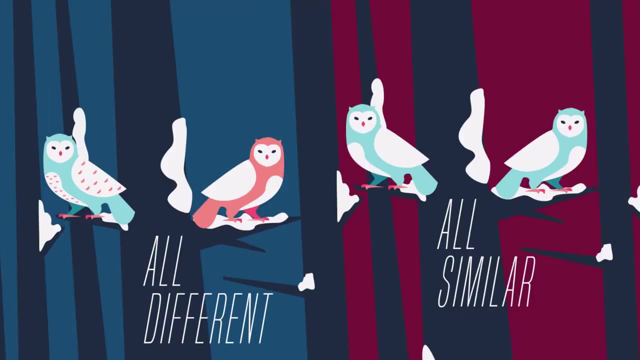 problem is that the key to having a healthy population is genetic variation. Within a population you need a large variety of different characteristics so that a species can adapt if there is a change in the environment and avoid becoming extinct. This can happen if all the members of the species have similar genes. 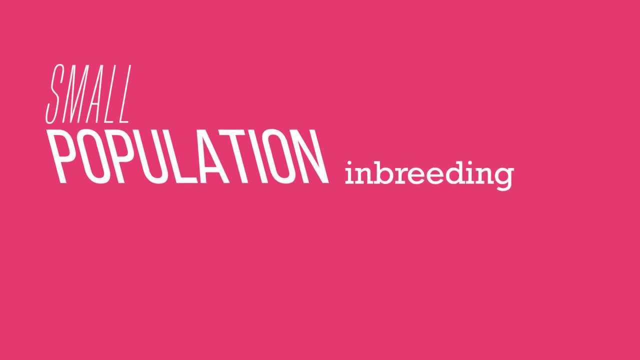 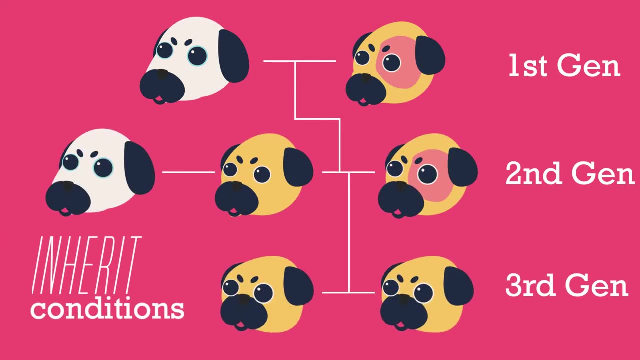 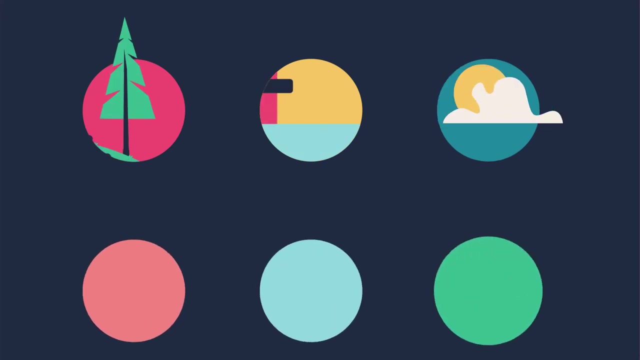 Also, in a small population, there is a high chance of inbreeding. where closely related individuals breed, this can increase the risk of offspring having inherited conditions. so large wild populations are important for a species survival. there are many reasons why a species might become endangered. it can happen because of habitat destruction, climate change. 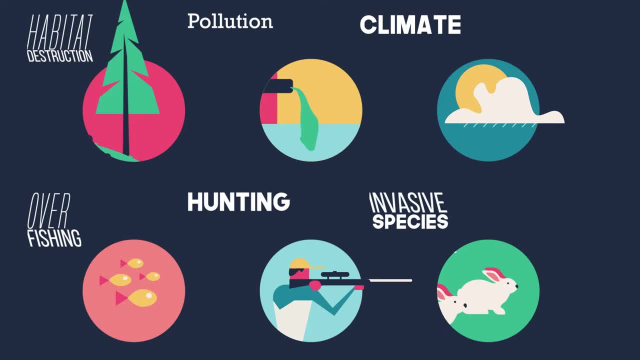 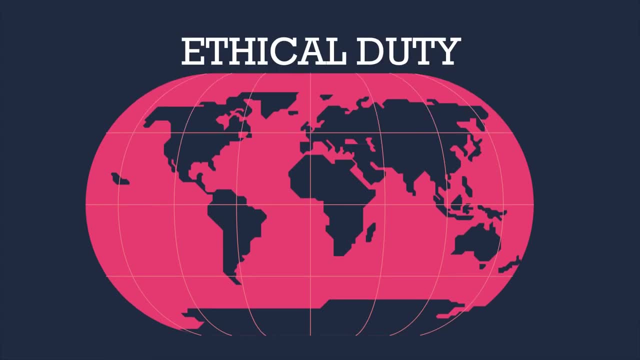 over fishing or hunting and the introduction of invasive species to habitats which outcompete the native ones. we have an ethical duty to help preserve all the species on earth, and this is done by carrying out conservation. let's look at a few methods used. firstly, endangered animals can. 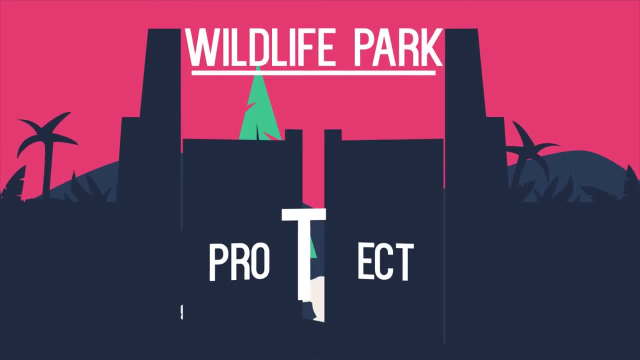 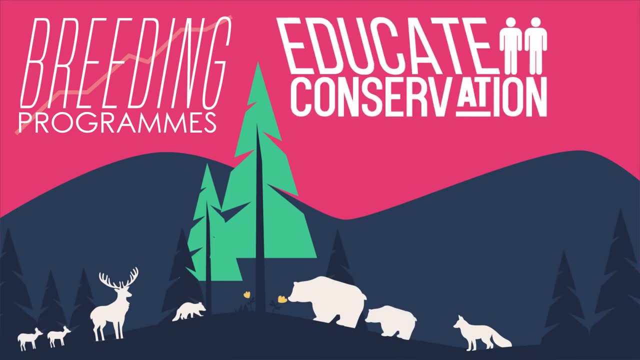 be housed in wildlife parks. this protects them and also captive breeding programs can be used to increase their numbers. they help educate people about conservation and how we can all help protect endangered species. they also help the general public to form an emotional connection to these endangered species. however, 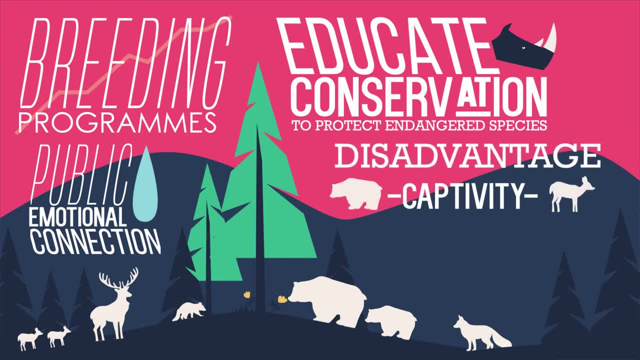 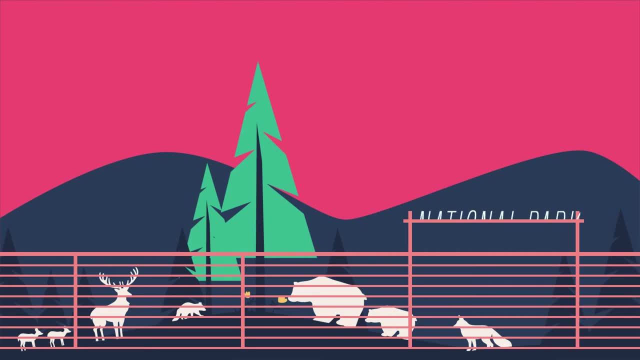 there are disadvantages to animals in captivity. the animals do not lead a normal life and there is risk of inbreeding. a way of protecting animals in their natural habitat is by creating protected areas like national parks. trees cannot be cut down, roads and houses can't be built and hunting 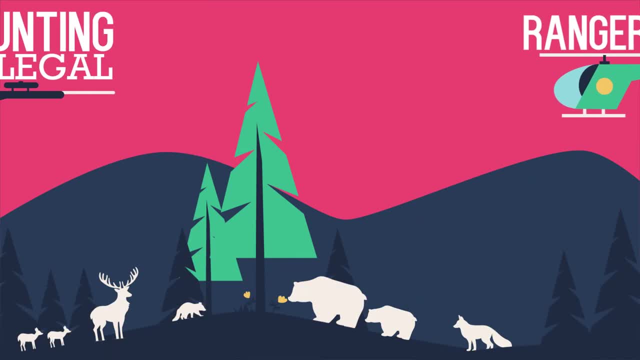 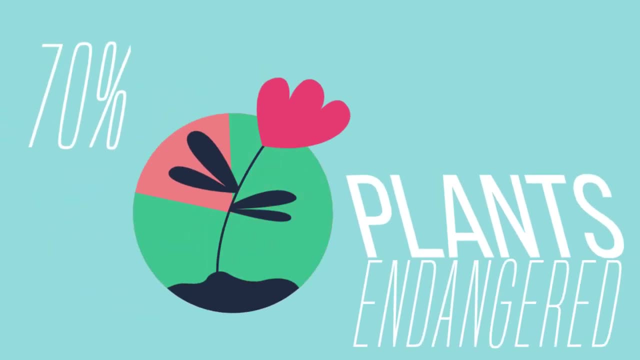 of the animals is illegal. rangers are employed to make sure this is enforced. it's not just animals: plants are also at risk. an amazing 70 percent of plant species are endangered. so it's vital that we help protect the animals. we can't just keep them in the wild. we can't just keep them in the wild. 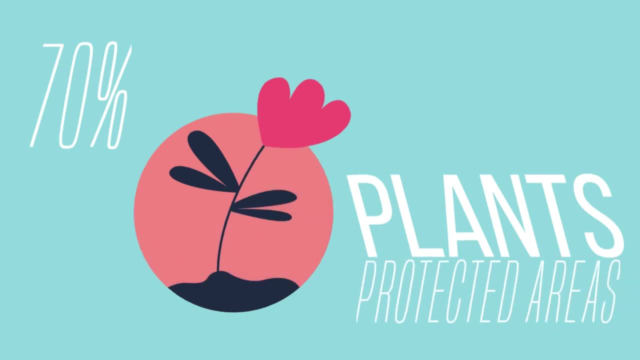 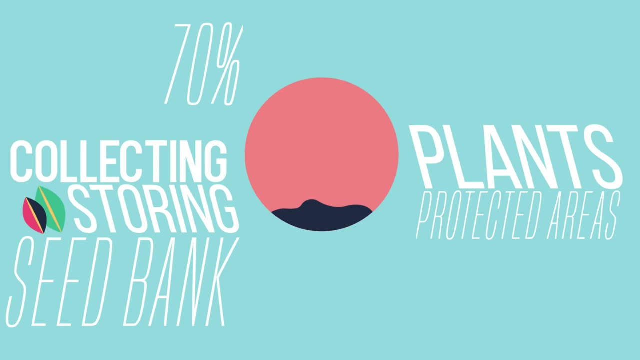 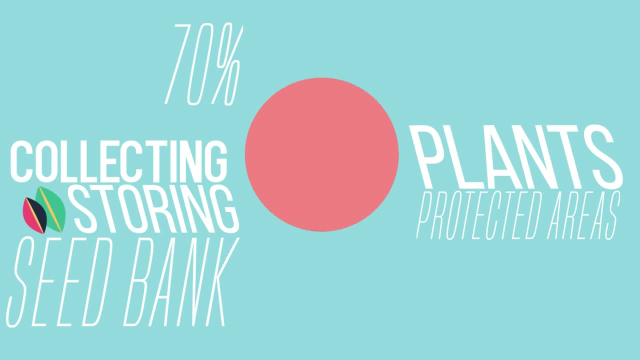 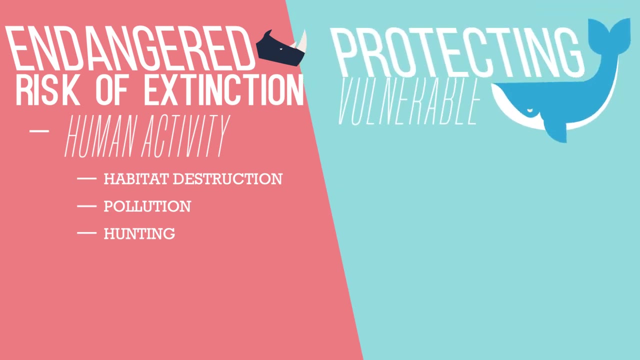 restore their populations. to recap, an endangered species is one that is at risk from extinction, the main causes of which are human activities. protecting vulnerable species is called conservation, and there are many methods to do so, including wildlife parks and protected areas. if you liked the video, give it a thumbs up, and don't forget to subscribe to our channel so you don't miss our next video.